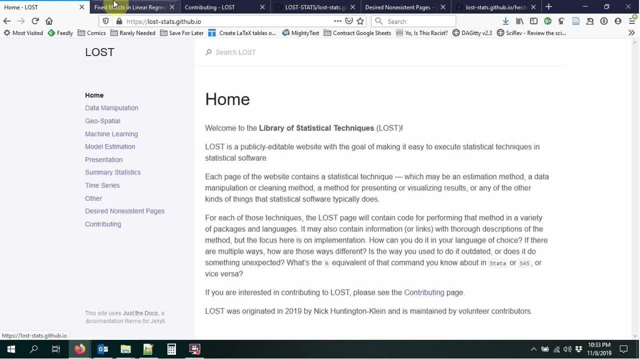 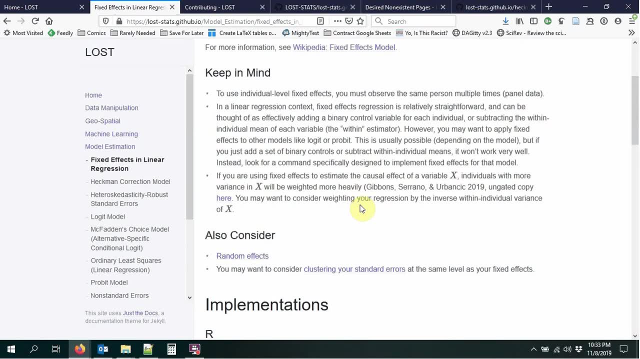 doing data visualization and other kinds of presentation of your data. Each LOST page contains all sorts of useful information, including information about the method that you're trying to perform, things like assumptions that you should be keeping in mind when you are performing that statistical technique and other interesting techniques that you might want to. 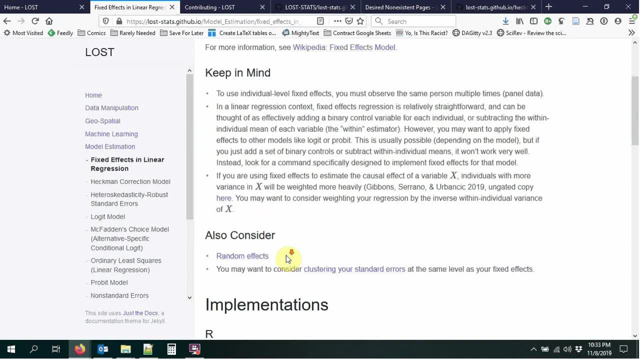 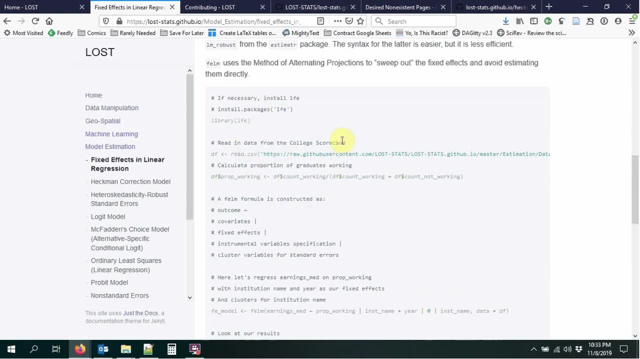 think about using in addition to or instead of whatever you are currently trying to do, as well as examples of performing this technique in code that you can use to get at things running yourself. LOST is publicly editable, meaning that we're always looking for people to help contribute. 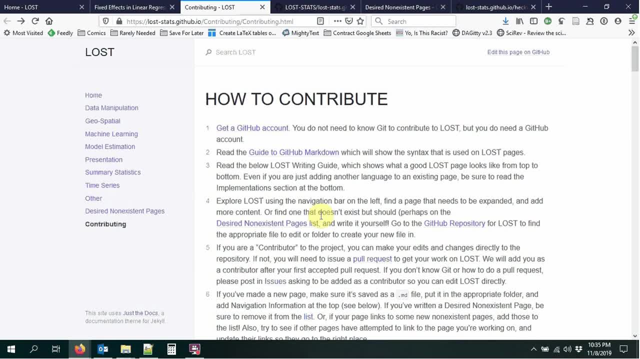 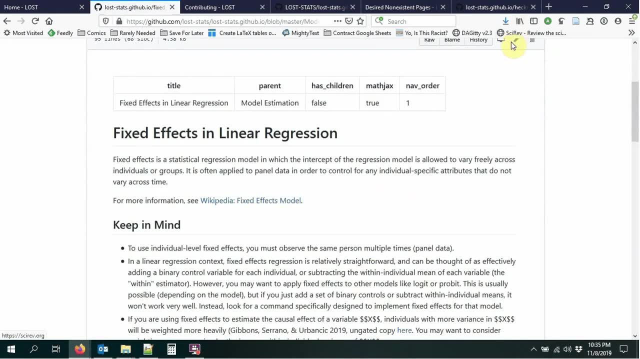 and add the knowledge that they have to pages that already exist or write entirely new pages of their own. On any page, you can click the edit button and then click the edit button. You can edit this page on github link in order to find the text file that you can just edit directly. 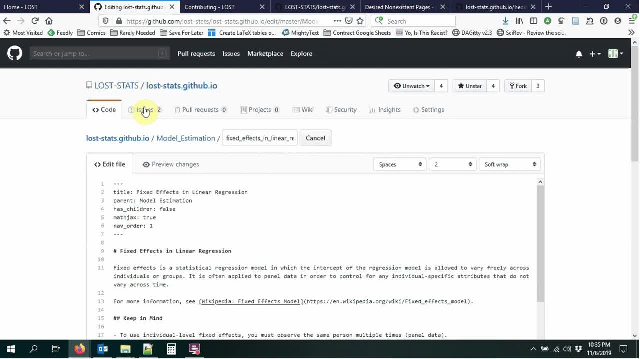 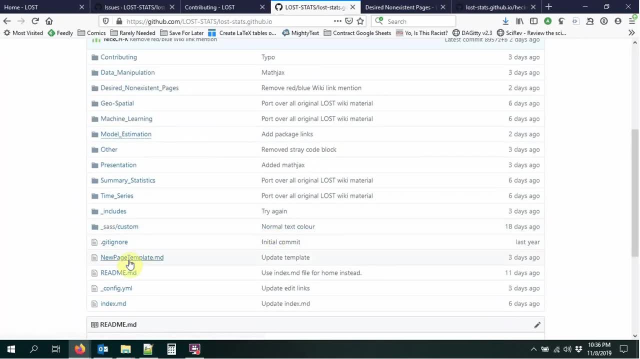 yourself as soon as you become a contributor, which you can do very easily by asking to become a contributor on our issues tab. You can also go to our github repository directly and write a new page using our new page template. There's always plenty of pages that we're looking for help. 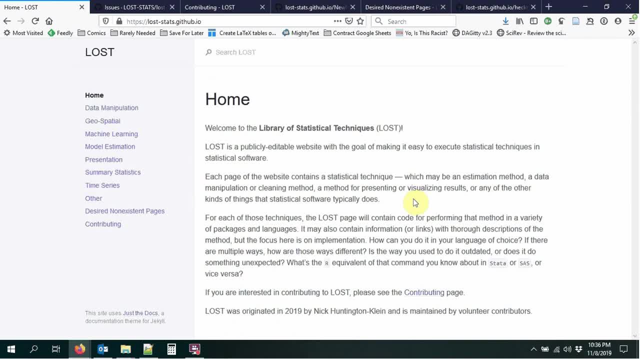 writing. Using statistical software can be difficult. LOST is here to try to help you figure out how you can perform the techniques that you're trying to do in whatever language you're interested in. We hope you enjoyed this video and we'll see you in the next one. Bye. 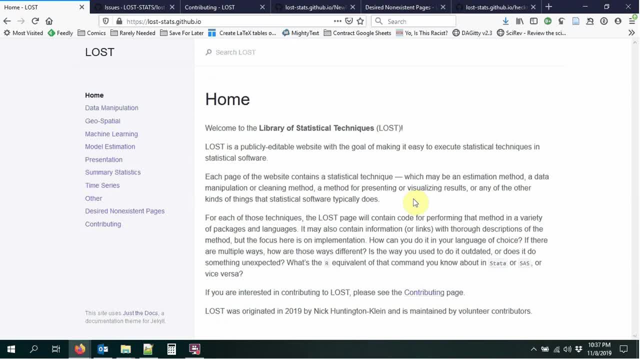 I hope that you find it useful and maybe you'll find the time to be able to contribute as well. Thank you. 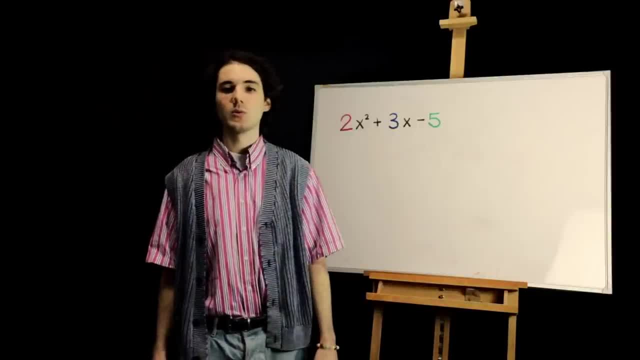 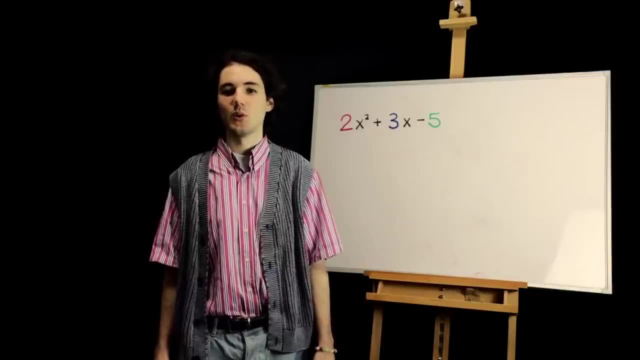 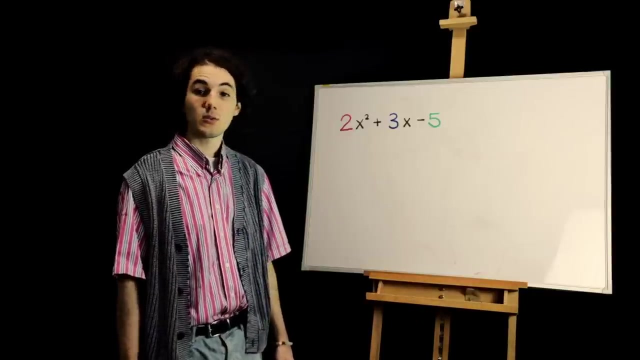 Hello and welcome to Monday Math with Martin. It's Monday, I'm Martin and this is math. In today's show, we're talking about polynomials Like this one: 2x squared plus 3x minus 5.. Now, if I ask you to find the roots of this polynomial, I trust that you will know what to do.